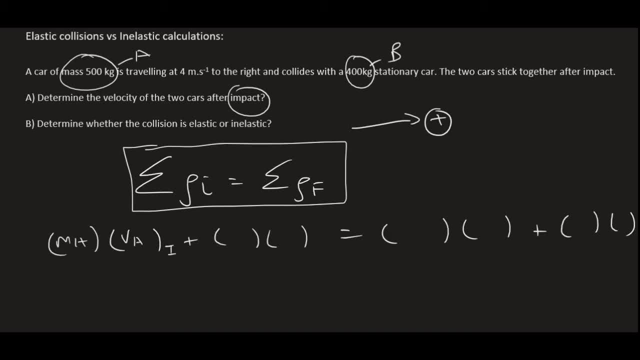 mass of A. velocity of A. and then I'm going to put an I for initial, or I could use small letters, I doesn't really matter. and then B and velocity of B: initial. mass of A. velocity of A final I. 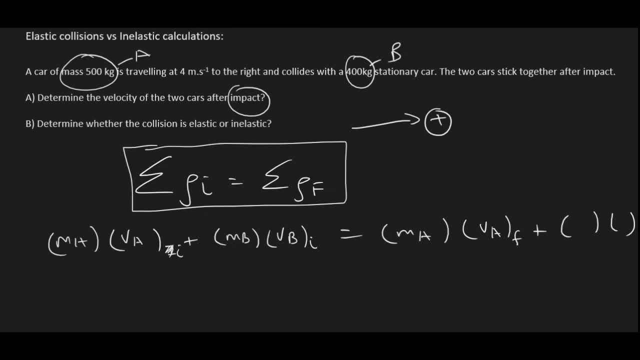 hope that now you know how to use this formula really easily or quite comfortably. and then mass of B, velocity of B and final. Now we just fill things in. So mass A is 500, its initial velocity is 4, the initial mass of the car B is 400, but it's not moving because it's stationary. 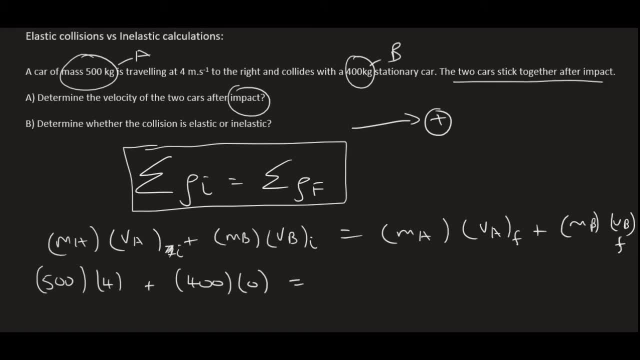 They say the two cars then stick together. so here your teacher might do some like type of factorizing thing over here, or they'll tell you to just make one big bracket. You don't have to, it's your choice. okay, So I'm going to keep it. 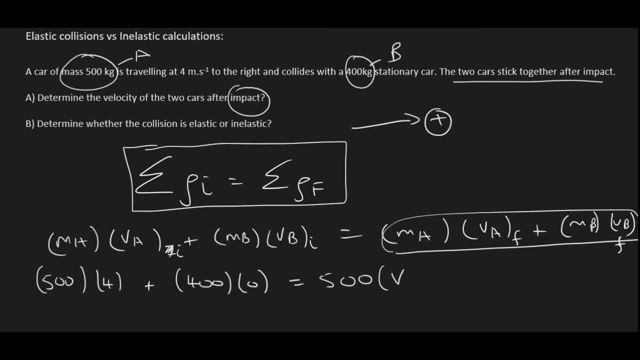 separate. so the mass of the first one is 500, but I don't know what its velocity is. I'm just going to call its velocity V, because I know that the 400 kilogram car is going to have the same velocity. Why do I know that? Because they stick together, and if two objects stick together, 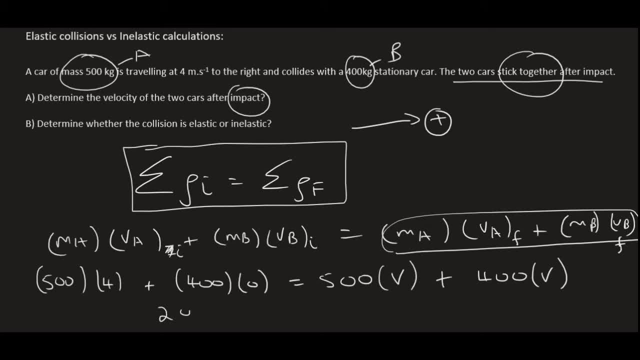 they will have the same velocity. On the left, we're going to end up with 2000, equals 2, and then 500 plus 400 is 900 V. The reason I can put them together is that their Vs are the same. okay, Always make sure that that is the case. and so we simply divide by 900,. 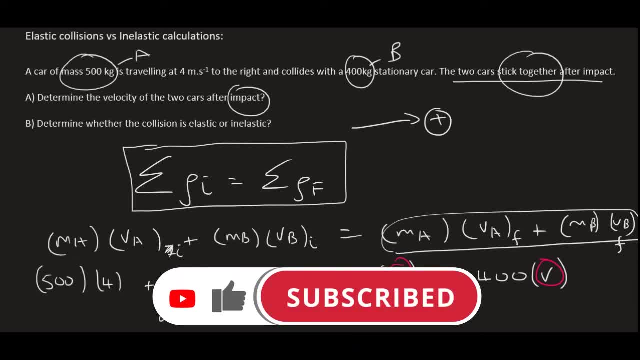 and so, therefore, velocity of both of those objects is going to equal to 2.22 meters per second. and because I got a positive answer and I chose right as positive, we're going to say to the right: Okay, so the first answer is 2.22 meters per second. 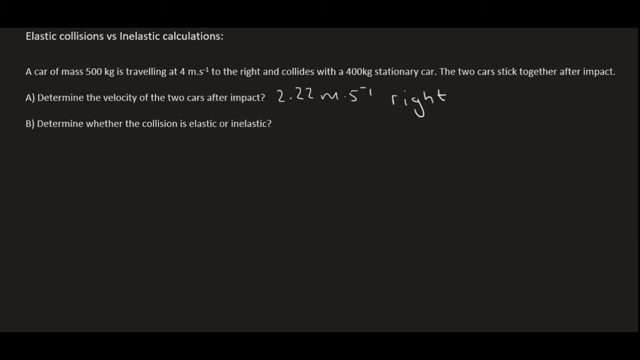 To the right. The next one is to determine whether the collision is elastic or inelastic. So to do that, we need to work out the initial kinetic energy, and so you just add up the energy. So, remember, kinetic energy is equal to a half mv squared. Remember the square And this formula. 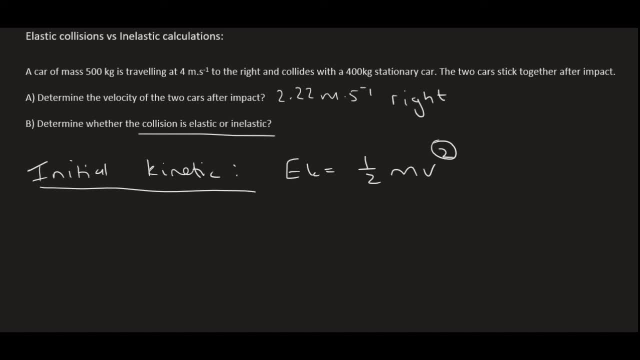 is given to you in the test, and so we can say the first object was a half and its mass is 500. It was initially traveling at 4.. Plus the second object, which has a mass of 400, but it was stationary. 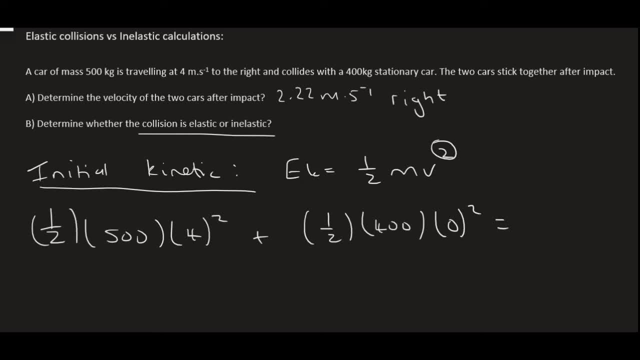 You can then type this all in on the calculator and you will get an answer of 4000, and the unit of energy is joules. Then I look at the final kinetic. Let me just write this nicely: Sorry, sometimes I write too quickly and then I leave out letters, as we saw in the previous video. 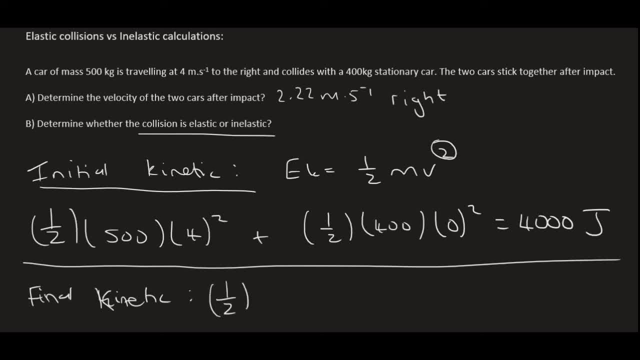 with energy. So here we've got a half. Now some teachers, because the two objects are together. your teacher might just say 900, you'd say 2.22 squared. see, i've combined all objects into one, but you can do it separately. 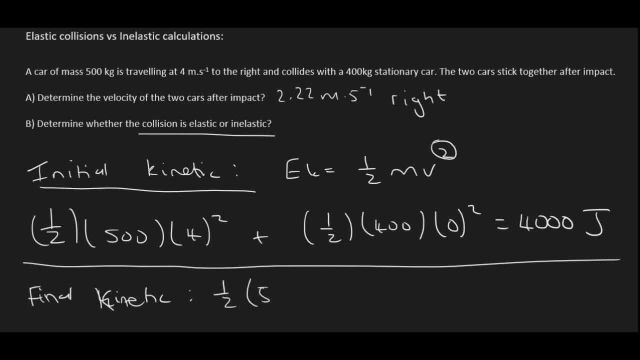 so you can do it like this: instead you could do the 500 kilogram object and it's traveling at 2.22 squared, and then you could simply add the other object which is also traveling at 2.22 squared. you must do whatever comfortable for you. you don't have to follow your teacher's method, if they ever. 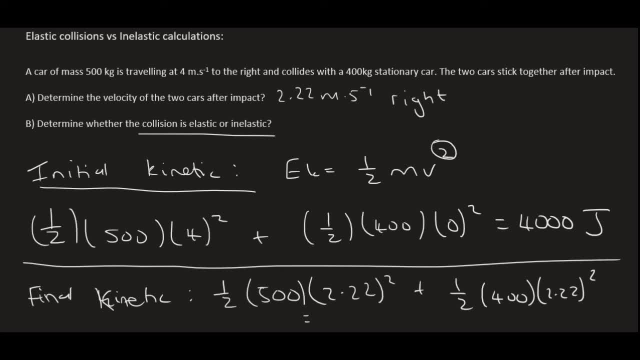 tell you to do that, just ignore them. you are allowed to use your own technique as long as it's comfortable for you, and so either way you do that. if you go type it in the calculator, you end up with 2217.78 joules. so the energy before is not the same as the energy afterwards. some of the 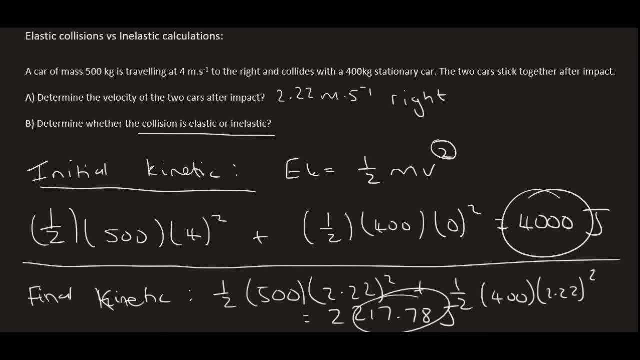 energy gets lost as sound and deformation, and so this whole collision is inelastic. what i see a lot of students doing for a question like b is they say that the energy or the kinetic energy, kinetic energy, yeah, the kinetic energy before. so they go: initial equals to the kinetic energy, final. and then they try solve it like that, guys. 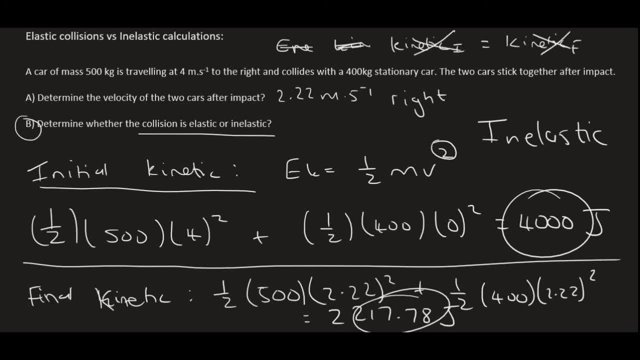 that's not correct. no one said that their kinetic energies are equal. you might be confusing that with the first formula, which says that the momentums are equal. the momentums are equal- that's a law that we know from physics- but no one said that the kinetic energies have to be the same. 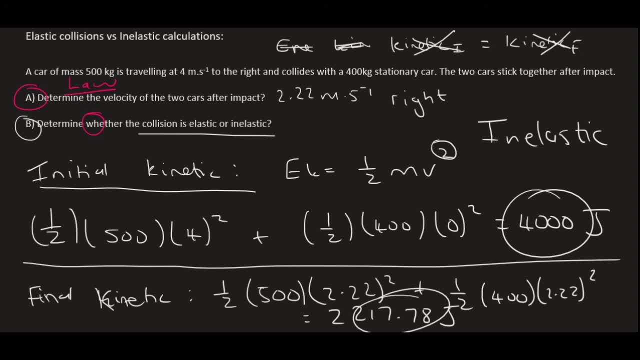 that might happen or it might not happen. you have to calculate each part individually, like this and like this, and then compare the numbers and see if it's the same.